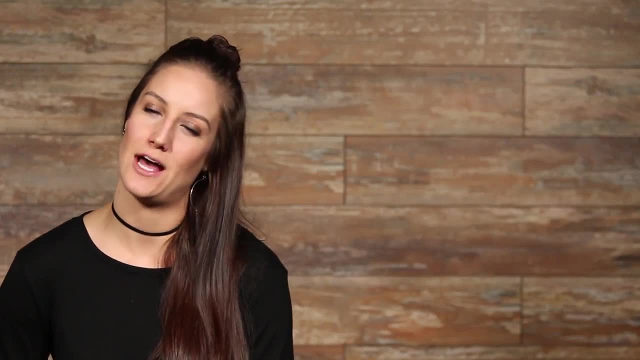 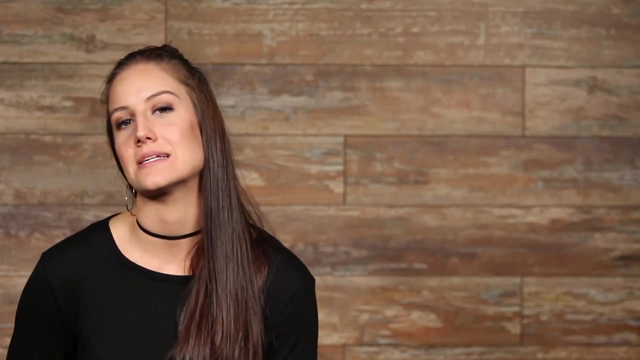 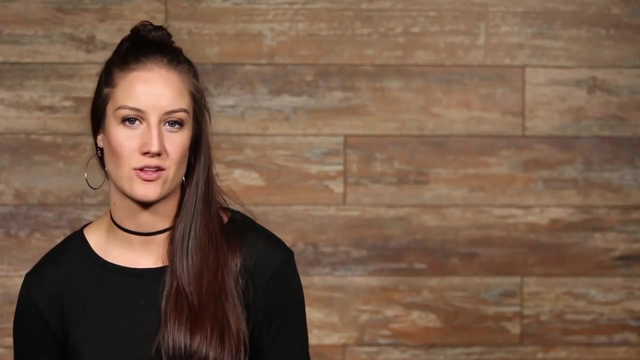 What I'm going to talk about in this video is a list of hints and helps Be advised. however, to really learn how to do word problems, you will need to practice, practice, practice. The first step to effectively translating and solving word problems is to read the problem entirely. 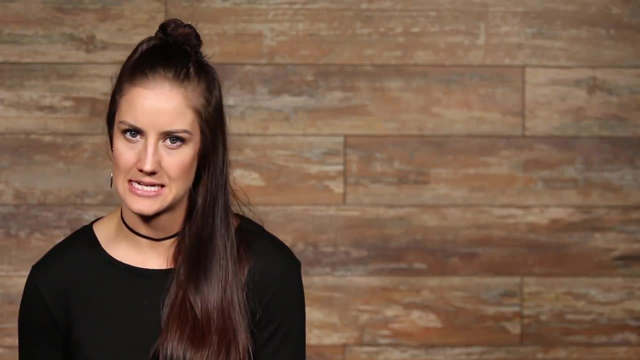 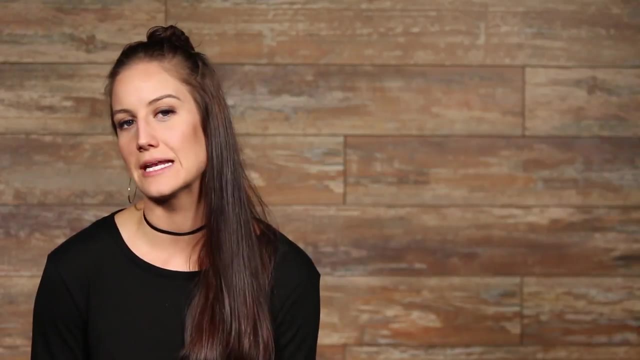 Don't try solving anything when you've only read half a sentence. Try first to get a feel for the whole problem, then see what information you have and figure out what you still need. The second step is to work on the problem. Work in an orderly fashion. 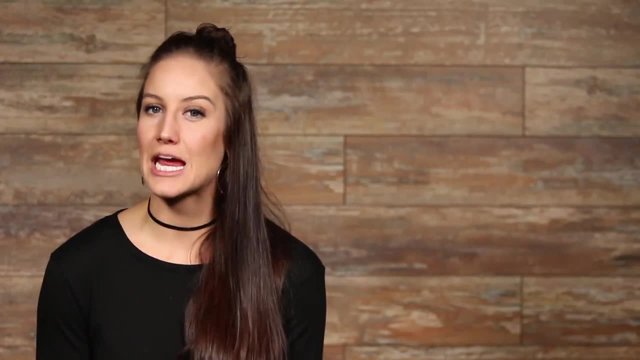 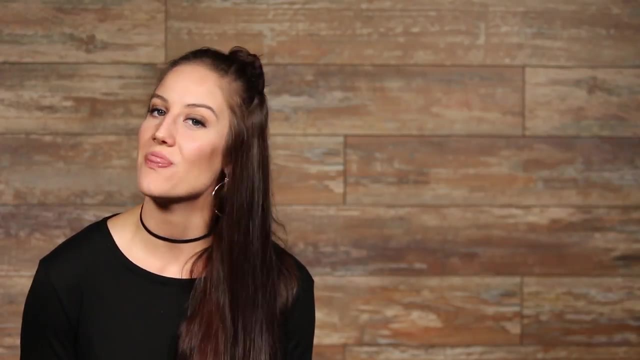 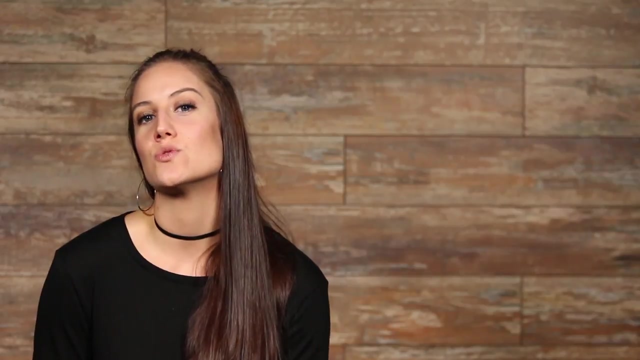 Figure out what you need, but don't have and begin to name things. Always pick variables to stand for the unknowns, clearly labeling the variables with exactly what they stand for. Draw and label pictures neatly, Explain your reasoning as you go along and make sure you know just exactly what the problem is asking for. 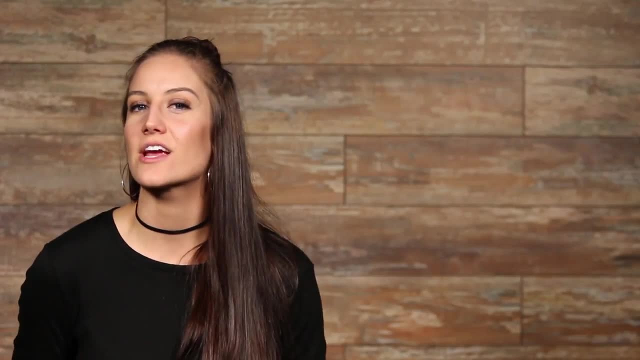 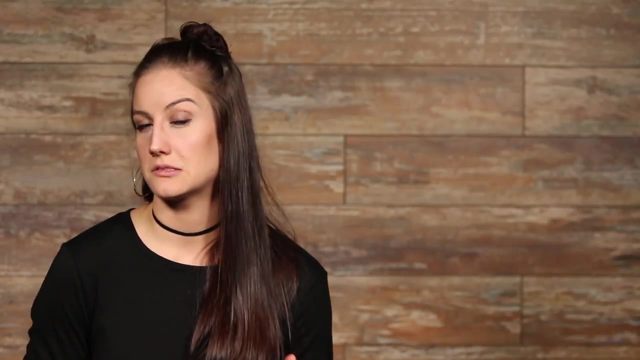 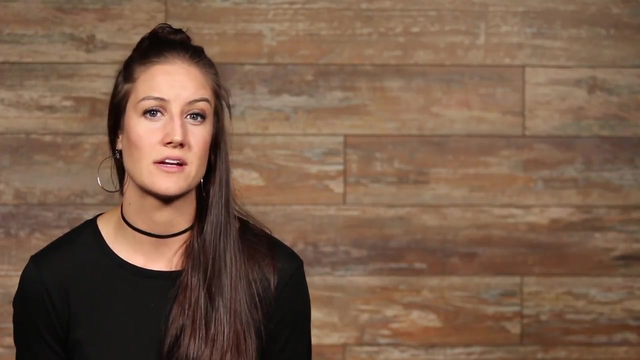 Working clearly will help you to think clearly, and figuring out what you will need will help you to translate your final answer back into English. It can be really frustrating and kind of embarrassing to spend 15 minutes solving a word problem on a test, only to realize that at the end you no longer have any idea what x stands for, so you have to do the whole problem over again. 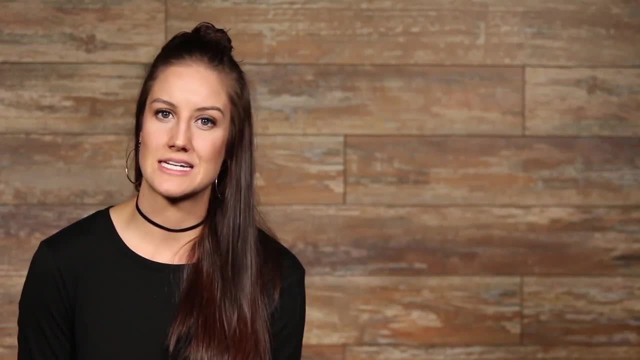 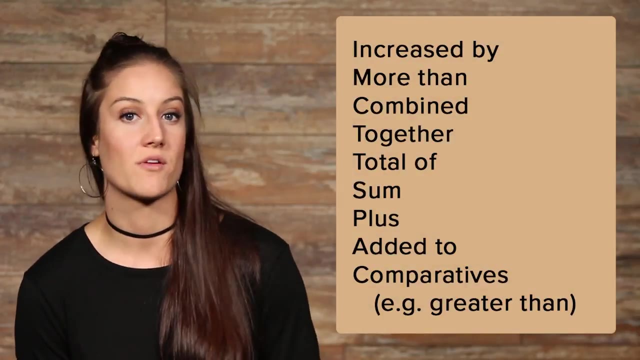 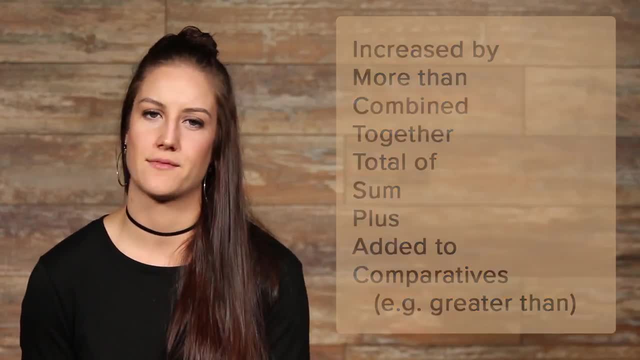 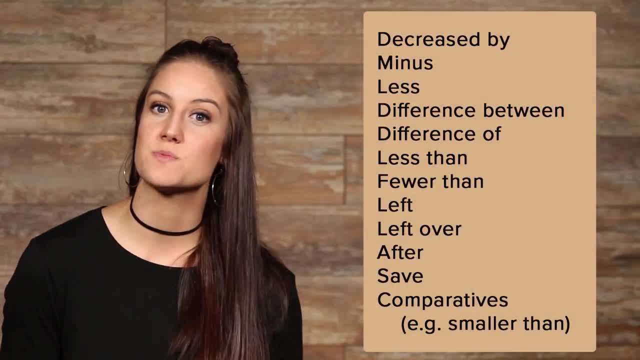 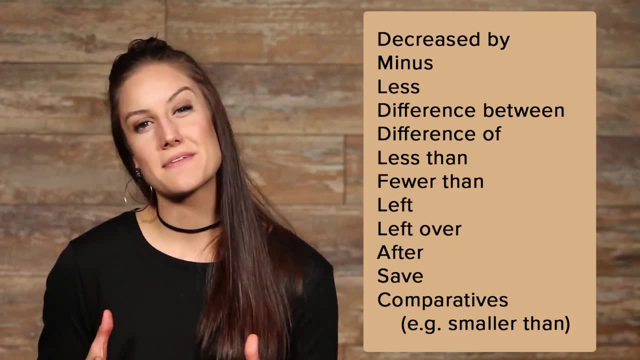 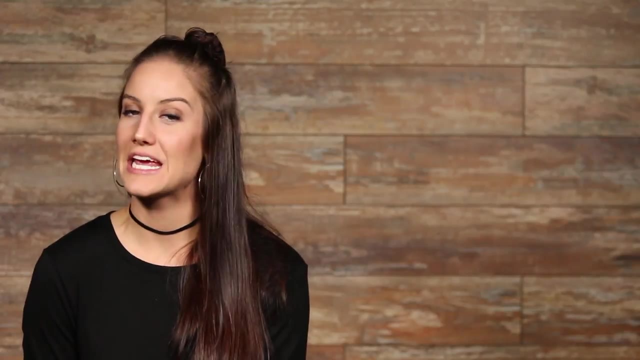 Decrease by minus less difference between, or difference of less than fewer than left, leftover after, or maybe even save, which is an old-fashioned term, And comparatives like smaller than Here are terms to be aware of when dealing with multiplication. 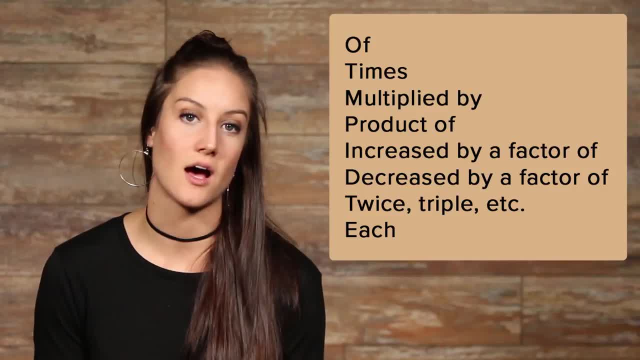 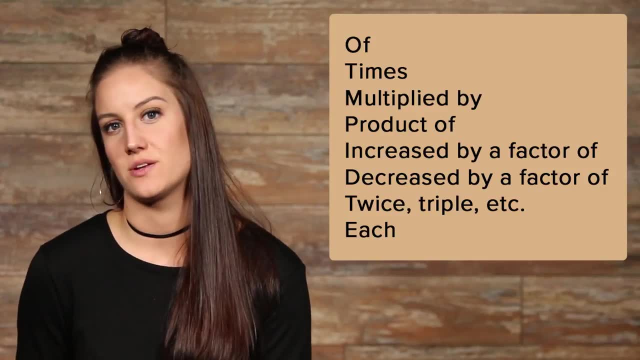 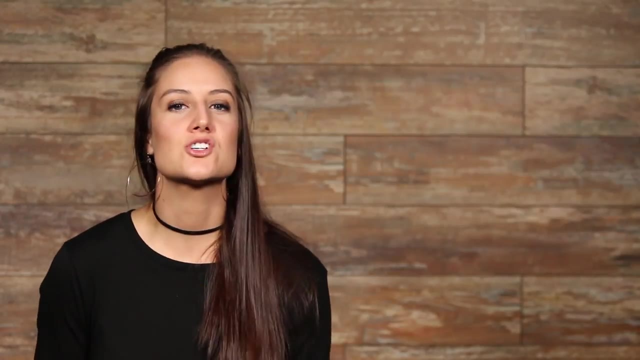 Of times multiplied by product of, Increased or decreased by a factor of, and this can involve both addition or subtraction and multiplication, Twice, triple, etc. and the word each. For example, they got three each. Next are terms to be aware of when dealing with division.